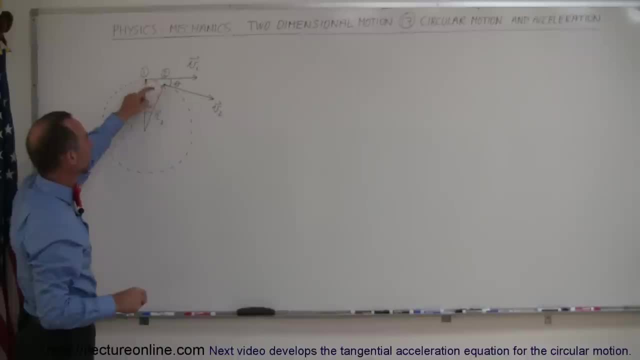 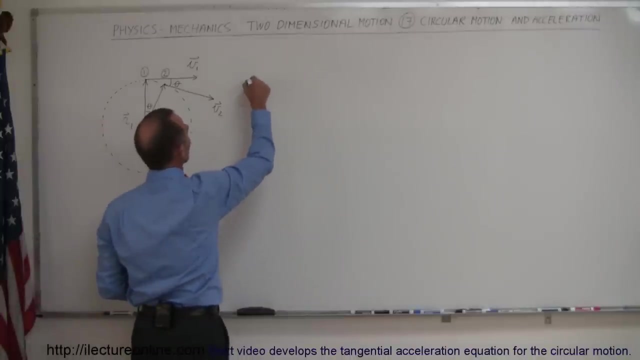 be the position vector of the object, based on the defined by the origin. for position number two, Notice that the angles between the two vectors must be equal to each other, and that's very important. Also realize that the definition of the acceleration can be described as the change. 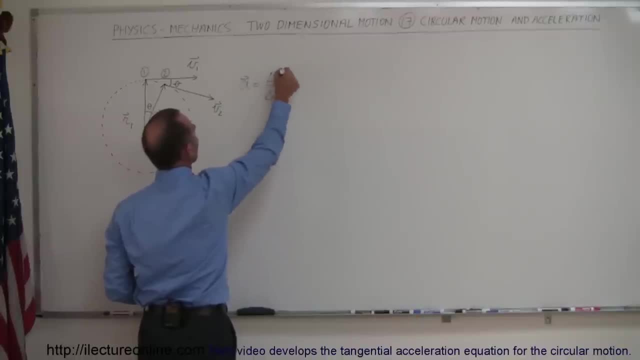 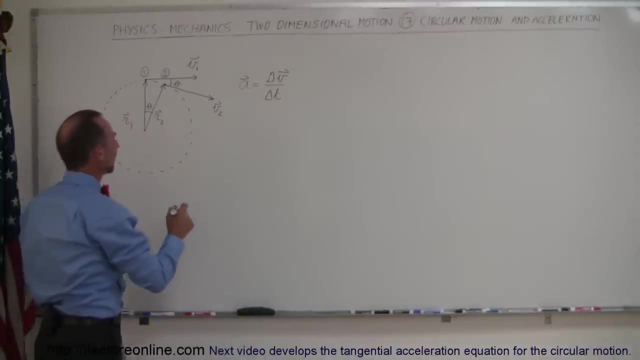 in velocity over the change in time. of course, if you make that vectors, it would be written like that: Now we can also claim, because the angles are the same, that the change in the position r over over the length of r must be the same as the change in the 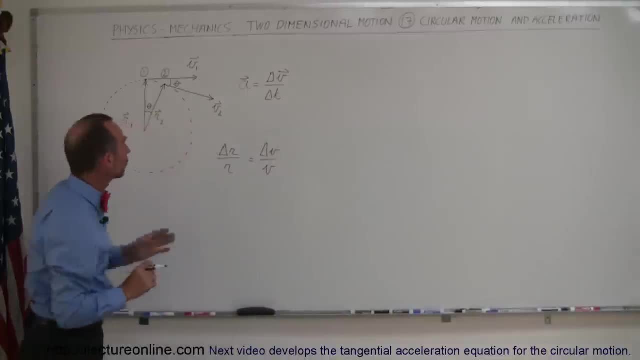 velocity divided by the actual velocity. so the ratio of the change, which would be this distance over that length, must be the same as the difference between the distance here, and of course I have to move this vector over here, so it would be the difference in the velocity vectors. 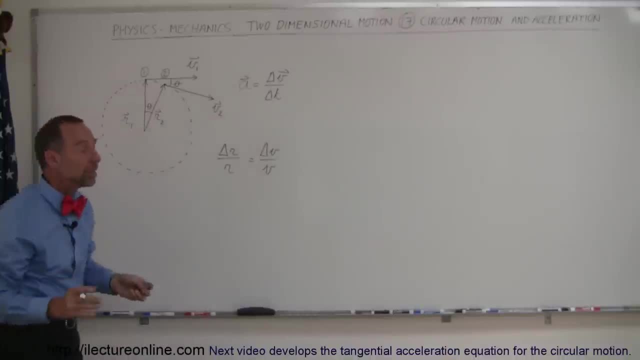 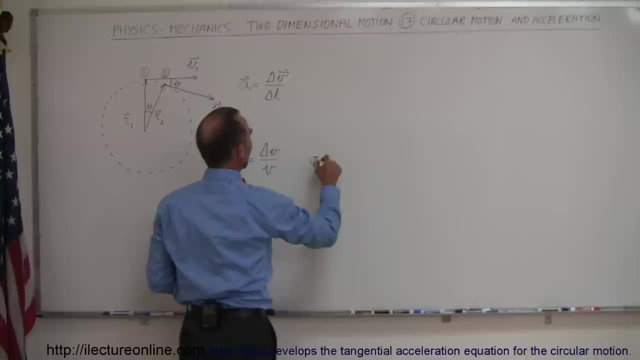 divided by length of velocity. they must be the same because the angles between the two vectors- sets of vectors- are the same. Also, I realize that I can write that the acceleration without the vector quantity is the change in velocity over time. so what I'm going to do is I'm 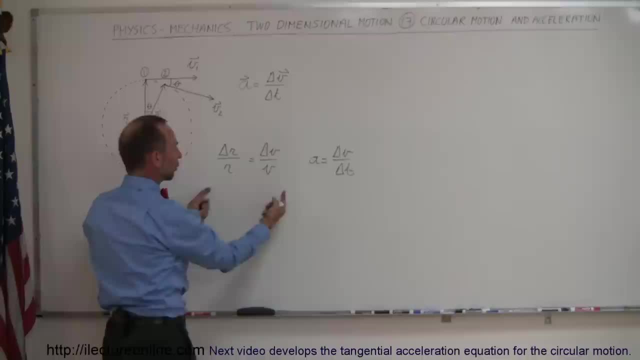 going to try and change this into that. so I'm going to rearrange this equation. I'm going to write this as delta v over v is equal to delta r over r. then I'm going to cross multiply, I'm going to move the v over here, so I now have delta v is equal to delta r times v over r. so simply, I'm going 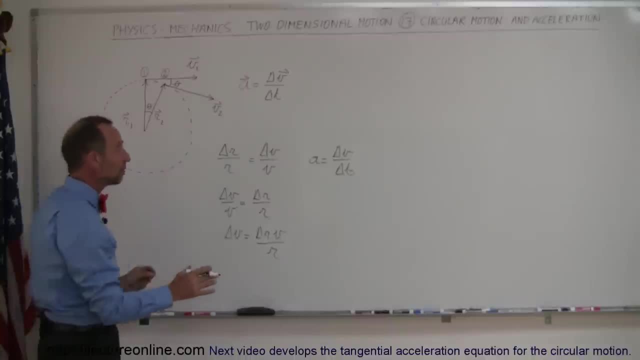 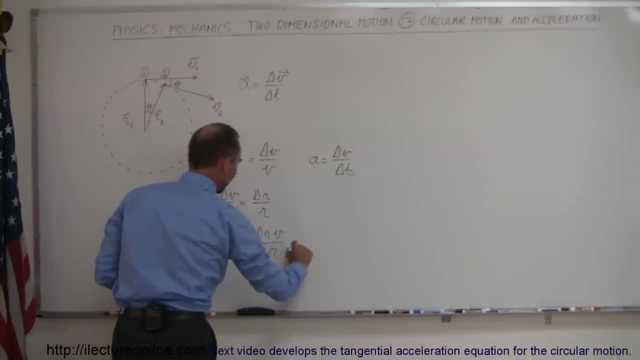 to move the v over there and I'm going to divide both sides of the equation by delta t. of course I do that to make it look like this. so I'm going to divide the left side by delta t and I'm going to divide the right side by delta t. all right. now that I've done that, I can say: well, this is equal. 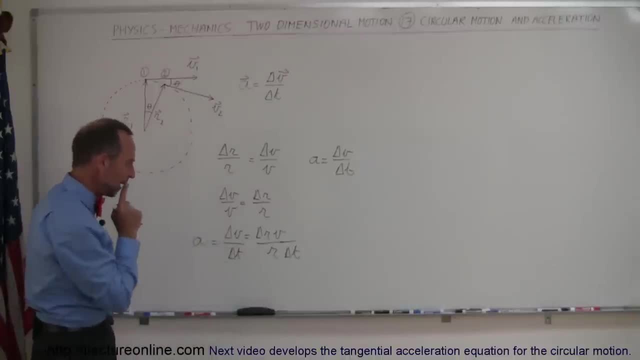 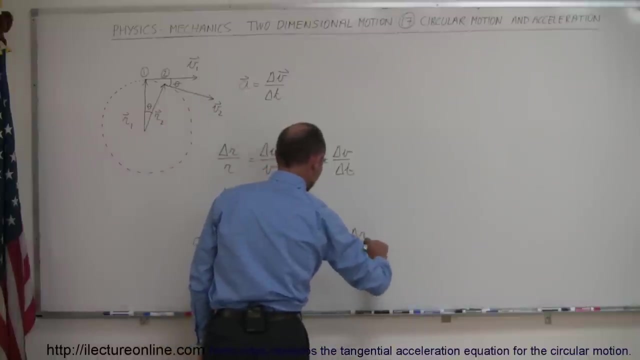 to the magnitude of the acceleration. so now what do I have here? I have v divided by r and delta r over delta t. so I'm going to rearrange that a little bit so it looks a little cleaner. so this can be written as v divided by r times, delta r divided by delta t. now this right here: delta r.